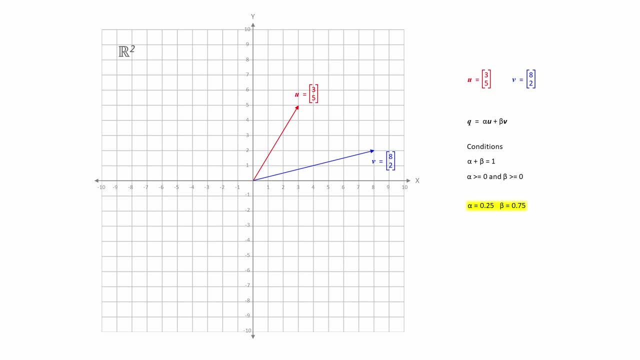 They add up to one and they are both bigger than zero. We can now substitute the vector coordinates and the coefficients into the equation, And when we perform the calculation, we produce a new vector, q, the tip of which lies on the line segment connecting the tips of u and v. 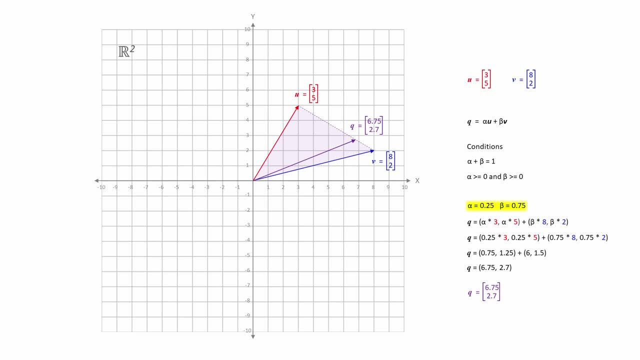 Notice that the line segment connecting u and v has been split in the same proportions as alpha and beta, namely 0.25 and 0.75.. Let's see another example with the same vector, q and the tips of u and v. 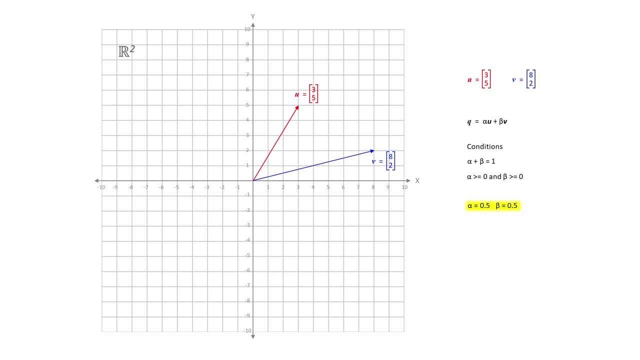 Notice that the line segment has been split in the same pair of vectors. This time, alpha is 0.5 and so is beta. As before, they add up to one. When these coefficients are substituted into the equation and the same calculation is performed. 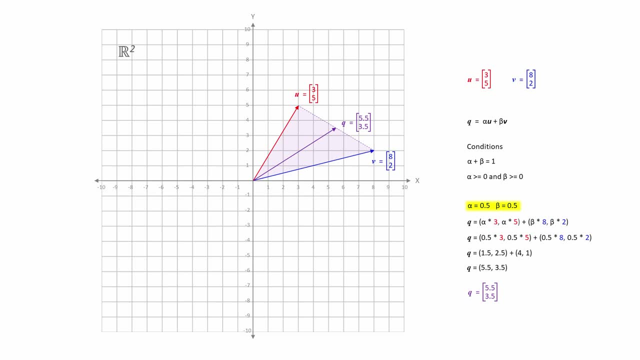 we generate a new vector with coordinates 5.5, 3.5.. Notice that this vector also splits the line segment in the same proportions as alpha and beta, namely in half. Here's one more example with these two vectors. This time we'll split alpha and beta in the proportions one-third and two-thirds. 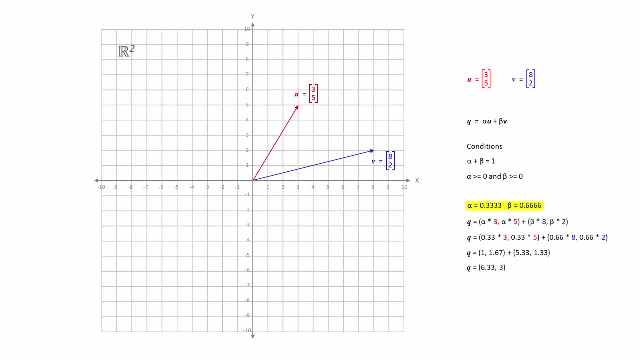 Strictly speaking, these values have recurring decimal places, so this time there will be some approximations in the calculations. Notice again that the line segment between u and v has been split in the same proportions as alpha and beta. And let's take a quick look at the line segment between u and v. 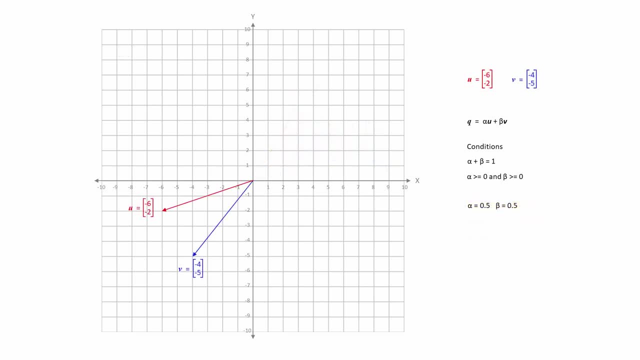 Take a look at a convex combination with two different starting vectors, This time u and v. both have negative coordinates. The coefficients are again 0.5 and 0.5.. As before, the tip of the new vector lies on the line segment. 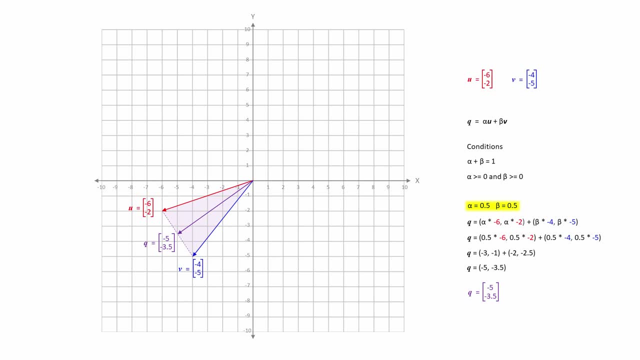 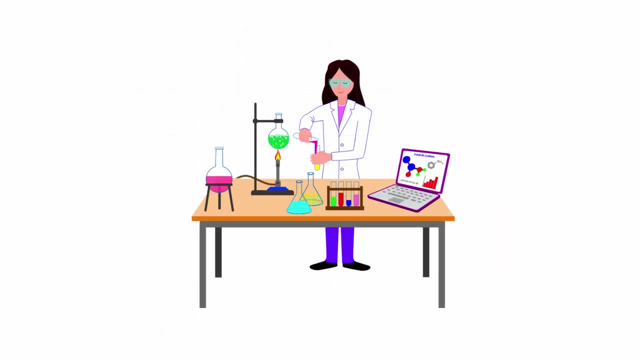 connecting the tips of u and v. Convex combinations have countless applications, including a few contracts between them. We're going to take a look at a нашей cannot count, but we're going to interesting number ofètres, rather unlikely ones, For example in the field of metabolic engineering. the